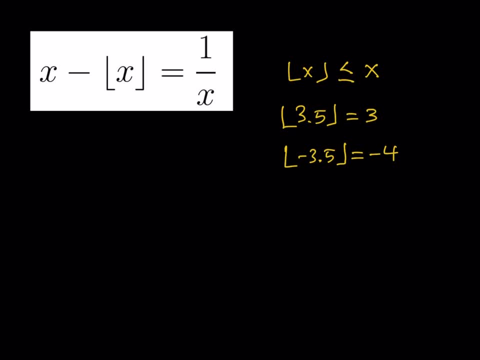 than or equal to x, Which means that this- on the left hand side we do have a positive quantity, Which means that on the right hand side we also have a positive quantity, Which means 1 over x- is actually non-negative, Since x cannot equal 0, we can safely say that 1. 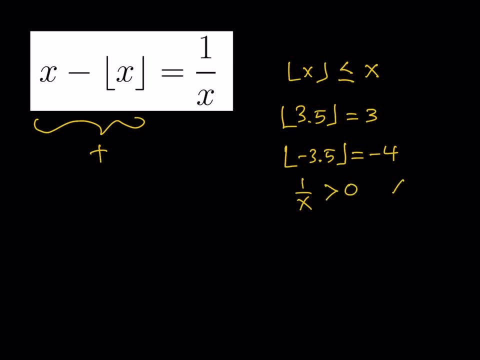 needs to be greater than 0 or x is greater than 0. Since x does not equal 0, we can safely say that x must be positive. So let's take that into consideration as we solve this problem. Now, how do we solve this problem? Well, one of the things we can do, which is kind of fairly nice, is: 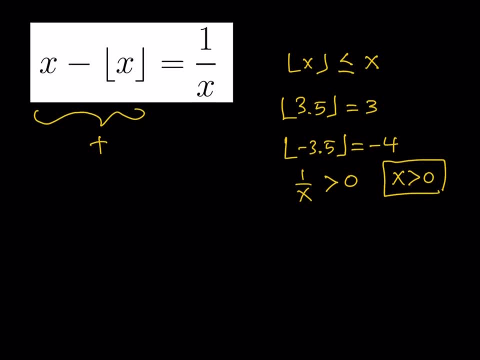 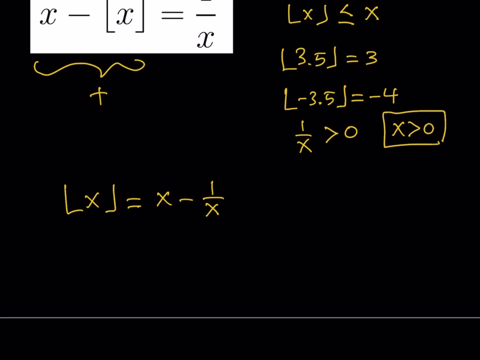 let's isolate the floor value of x here, So we can write it as the floor value of x equals. if you go and put it on the right hand side and switch sides like this, you're going to get the following equation: So the floor value of x is going to equal x minus 1 over x, right, And then what you're going to do? 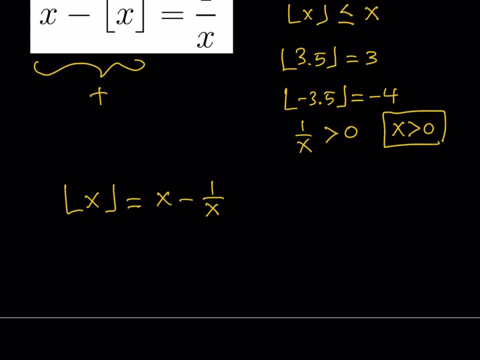 is most of the floor value. problems can be solved with substitution, So that's what I'm going to do here. Let me go ahead and call this n. All right? so by calling the floor value of x equal to n, we get an inequality. Since the floor value of x is the greatest integer function. this indicates: 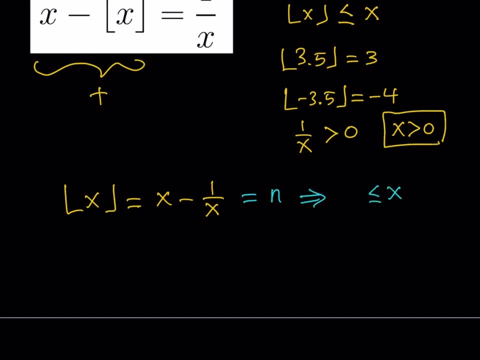 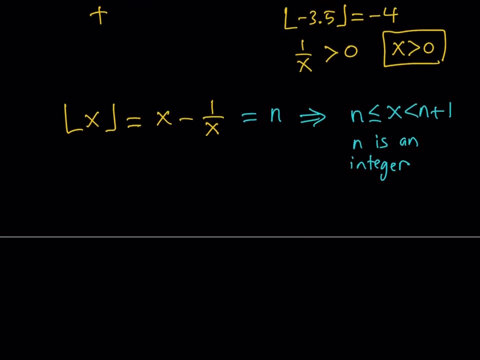 or implies that x must be between n and n plus 1, in which case n is an integer. Okay, n is an integer, x needs to be in that interval. So we're going to check that as well. Cool, now how do we proceed from this point on right? Well, 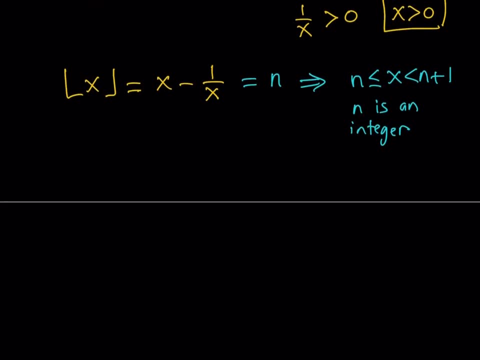 we do have like an equation here which we can use. Let's go ahead and write that down. So we have- I'm probably going to switch over here. Okay, x minus 1 over x is equal to n. Let's go ahead and multiply both sides by x, and obviously x does not equal 0.. We know that, we're. 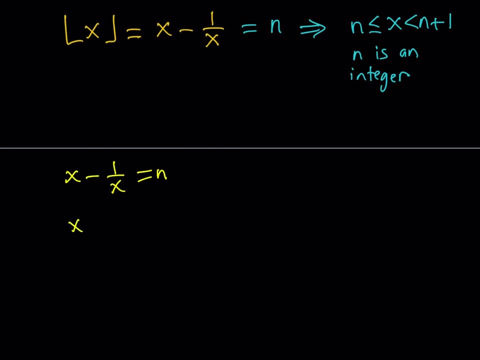 right. So it's okay to multiply both sides by x. That's going to give us x squared minus 1 equals nx. A lot of people try to make common denominators. You don't really need to do that. Just multiply both sides by the common denominator and you'll get a nice expression. 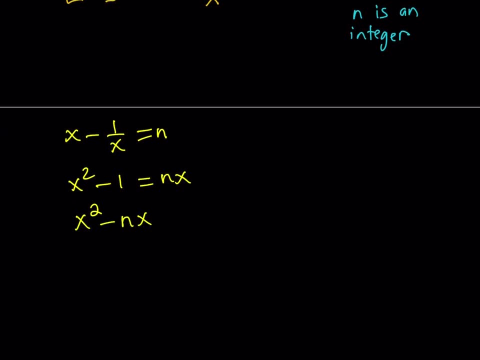 So let's put everything on the same side: x squared minus nx minus 1 is equal to 0.. So what do we get? n is an integer and this is a quadratic equation. So how do you solve this quadratic equation, Since we don't know what n is and n could be any integer, right Well? 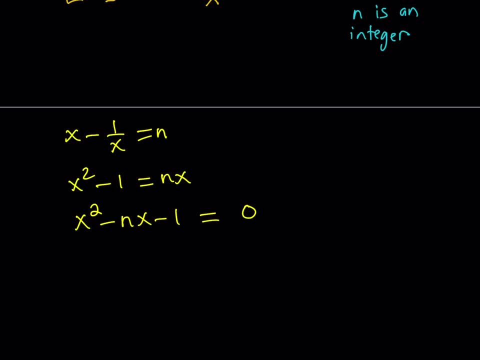 can just use the quadratic formula, right? I mean, since this doesn't seem to be factorable, So we can just go ahead and use the quadratic formula. Let's use it. x equals negative b, which is n plus minus the square root of b squared. In this case, it will be n squared. 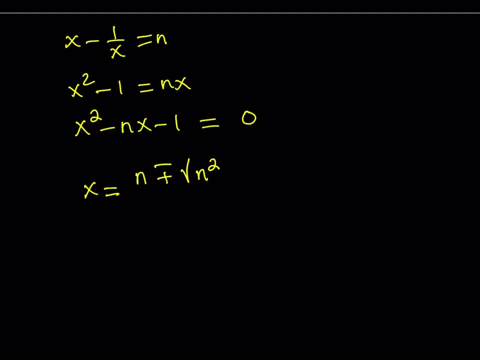 minus 4ac. A is 1.. C is negative, 1. So their product is going to be positive, 4.. And then we're going to get this and all divided by 2. Awesome, So we basically got the x value. 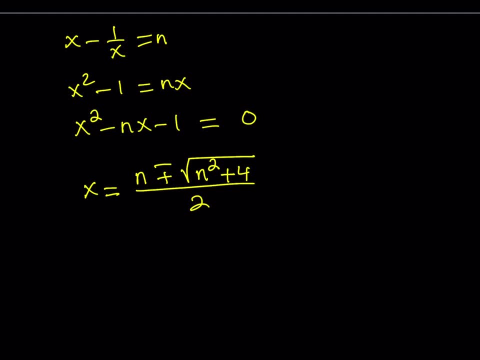 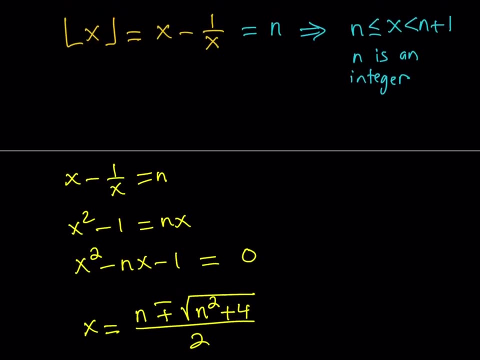 but it's not very specific. We're going to, you know kind of to talk about the details in a little bit, but before that i want you to realize one thing: here we actually started with some requirements, such as x needs to be greater than zero, right and n. 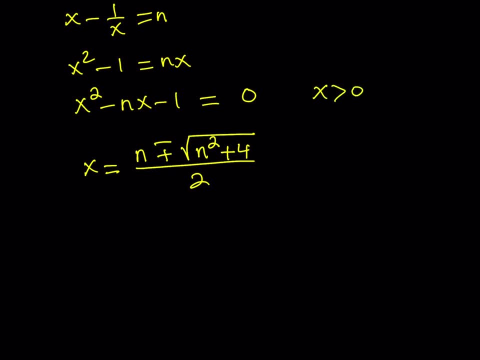 is an integer, so let's go ahead and copy those here. x is positive, n is an integer, so what's that supposed to mean? well, here, here's. here's something that i want you to realize. uh, first of all, let me go ahead and split these into two equations, because i need to look at them separately. 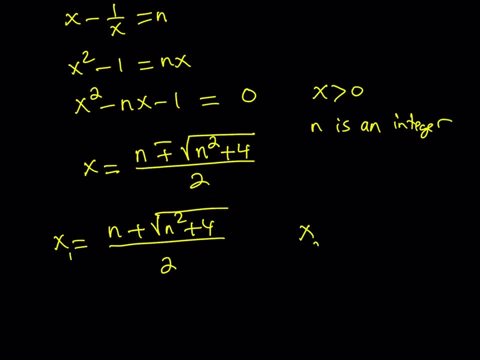 okay, there's going to be two solutions like x1 and x2: n minus the square root of n, squared plus 4 divided by 2. awesome, now take a look at each one of these separately. if you look at x1, is x positive here? well, n is an integer. if n is a positive integer, we're good. if n is a negative. 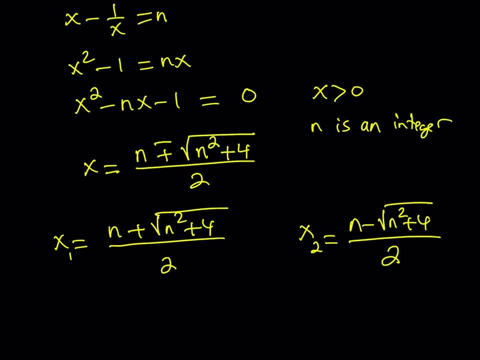 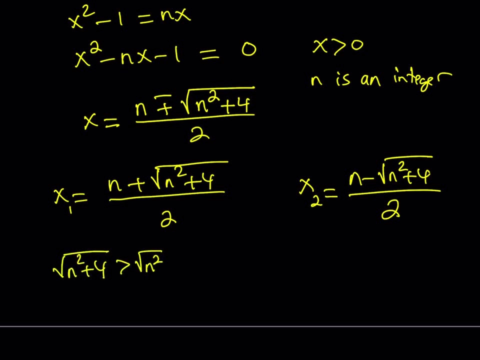 integer. we have to compare these two quantities. well, obviously, the square root of n squared plus 4 is greater than the square root of n squared, which is actually equal to n, right? so in this case, if n is a positive integer, this is going to work, but if n is a negative integer, if you think about, 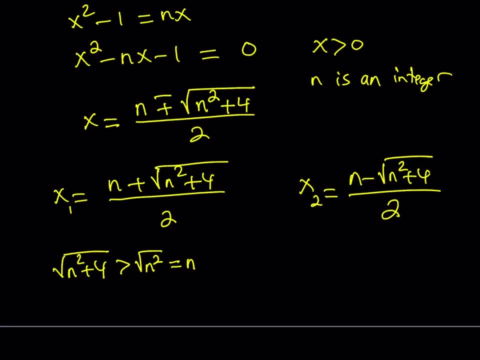 it. this is always going to be a positive quantity, right? and you subtract out, add a negative quantity, which is actually less than that. so this is always going to be positive. so the first one actually passes the test. but let's take a look at the second one. so we have a problem with the 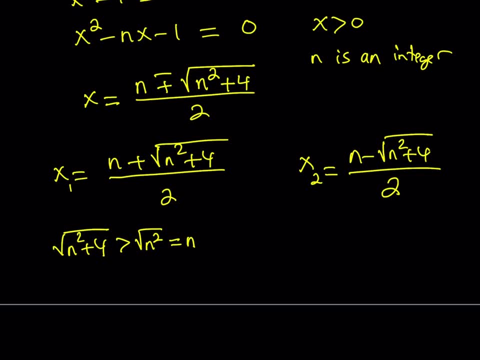 second one, because notice that the square root of n squared plus four is equal to xrien x squared plus 4.. greater than n, right? so this difference is going to be negative. so we're not going to be able to take the solution. we're going to reject it. okay, so we're going to go by the only solution that.